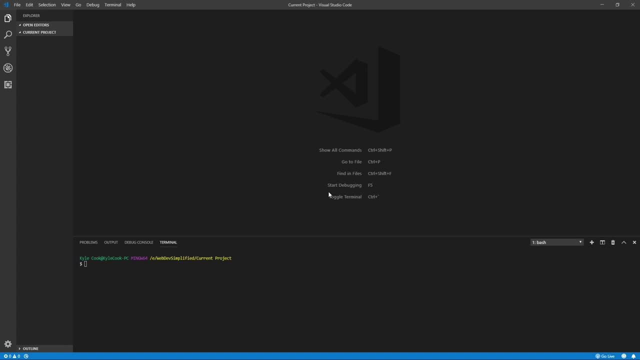 desktop apps, servers or really anything else that you want to do with JavaScript, and the thing that we're going to do is actually create a web server using Nodejs. So to get started with that, all we need to do is create a JavaScript file inside of our project, and we can. 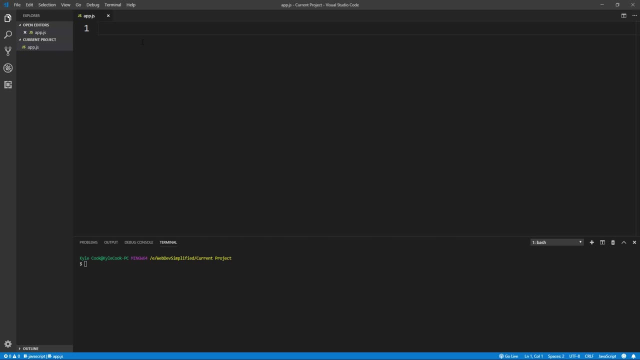 just call it whatever we want. In our case, we're just going to call it appjs, and inside of this JavaScript file, we need to create our server and tell it to start listening on a certain port. So the first thing we need to do is we need to require a certain library called HTTP. 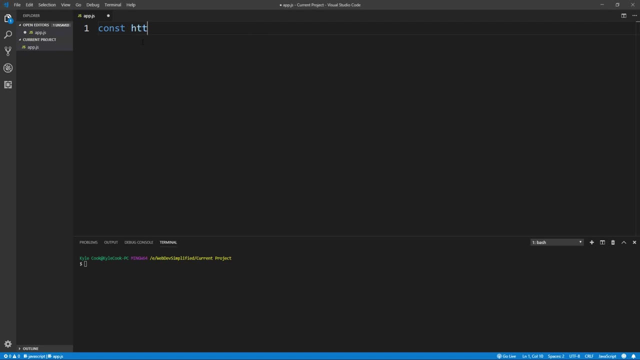 that is going to be used to start the server. So we can just create a variable called HTTP and to require a library in Nodejs you just type the require keyword, followed by the name of the library, which in our case is HTTP. 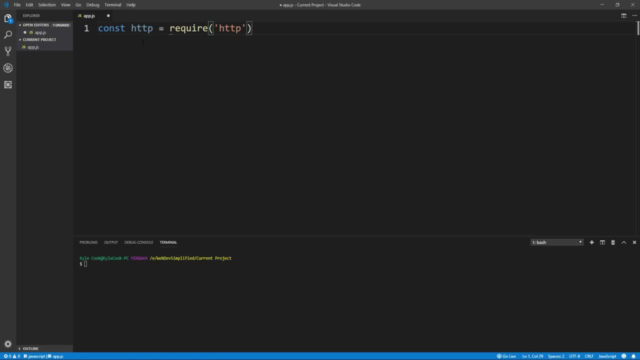 This will include the HTTP library into our code, inside of this HTTP variable that we created. The next thing we want to do is we want to create a variable that tells our code what port we're going to be listening to for our server, and we're going to use this later. 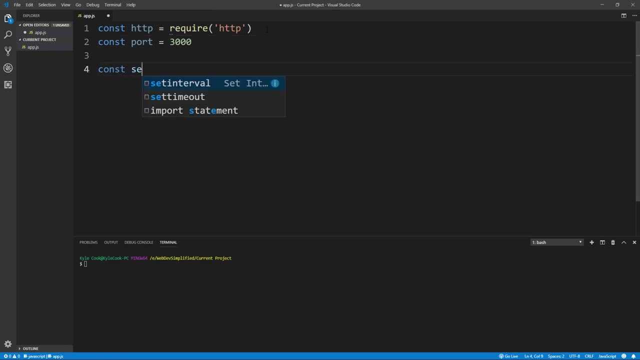 And then next we can actually create our server. So to do that, we'll create a server variable here and we're going to use the HTTP library we just imported and call the create server function on this object. And this create server function takes a single function that has two parameters. 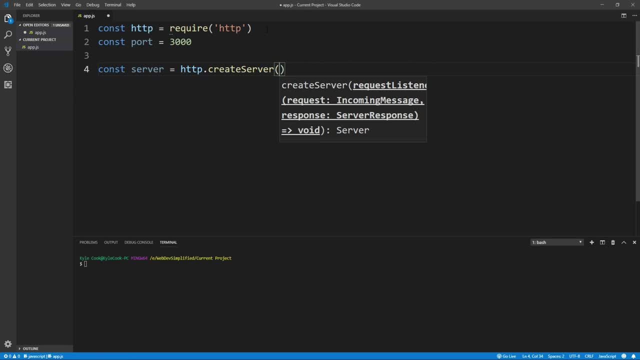 which is the request and the response parameters. So we just pass it in a function here with the request and response parameters, And then inside of this function is we're going to handle all of the different activity on our server. So every time someone requests a page on, 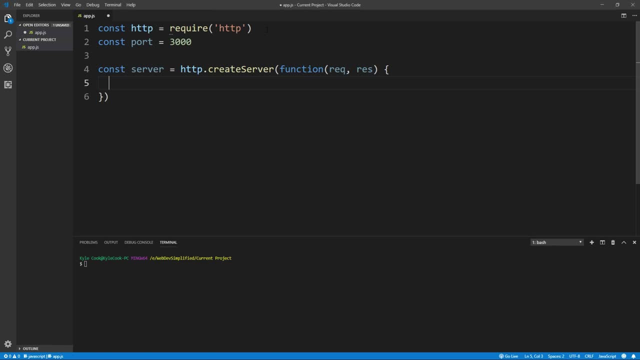 our server. it is going to call this function right here And we're going to implement this function in a little bit. The next thing we need to do is actually set up our server so it'll listen on the port that we want it to. So now that we have this server object, we can just call. 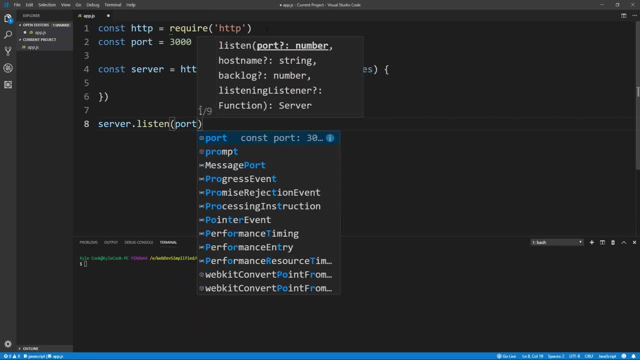 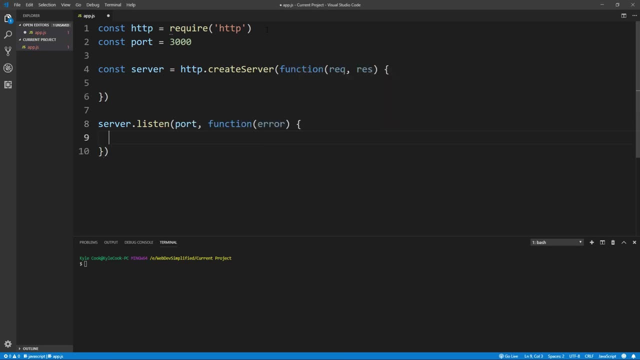 server dot listen, pass it that port variable that we created to tell it to listen on port 3000.. Then this takes a single function that it'll call if there's an error, potentially. So as soon as our server starts listening, it'll call this function and it'll either pass an error or nothing if it. 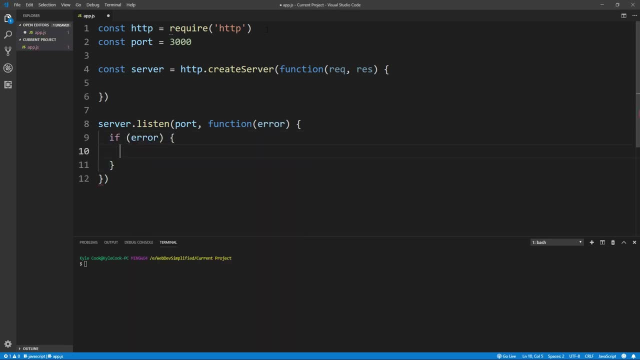 was successful. So we're going to check to see if that error exists, And if so, we're just going to log out a message saying that something went wrong, And then we're also going to pass the error along to that log statement so that when we check our logs we can see what the error was. that 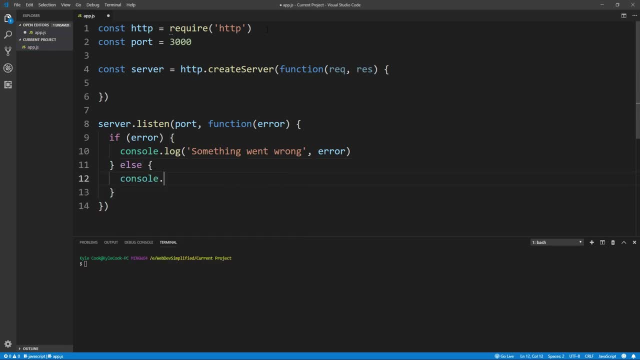 happened, But if there was no error, then we want to log that our server is listening on port And we're just going to pass in that port variable we created earlier. So now our server is actually listening And in order to run our server, all we need to do is type node followed by the name of the file we 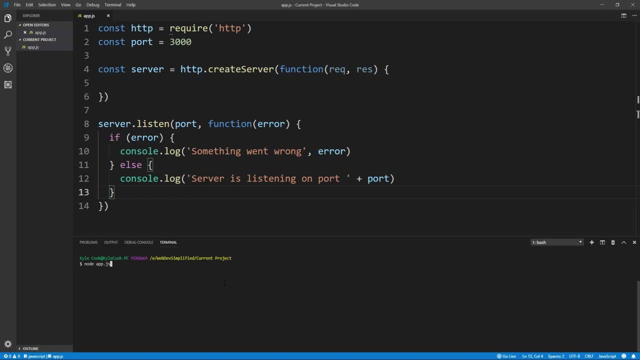 want to run And since our terminal is open inside of this project, we can just type node appjs And if we enter, you see, it'll say: server is listening on port 3000, which is perfect. But our server doesn't actually do anything because we haven't implemented the function inside of the create. 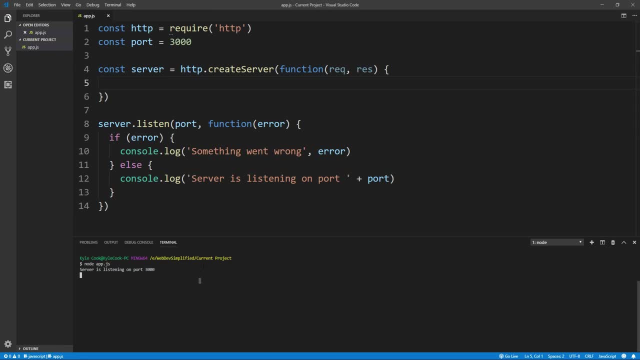 server function. So let's end our server by hitting ctrl C And then let's actually implement this function here. So what we want to do is we want to return some response to the user, And to do that we use the response object that has passed into this function So we can say response. 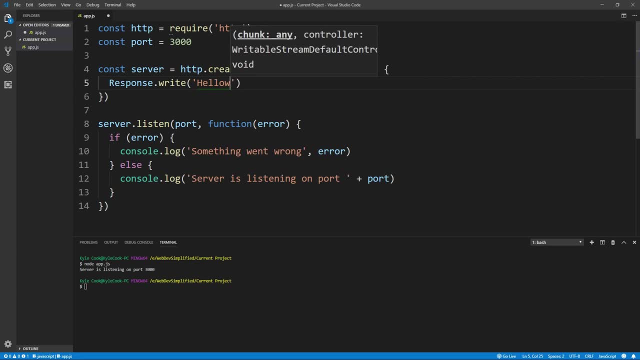 dot right and we just want to write hello node to every single person that requests something from our server. then when we want to end our response saying that we've written everything we want to write, we just type response dot end and there we go. that is everything. 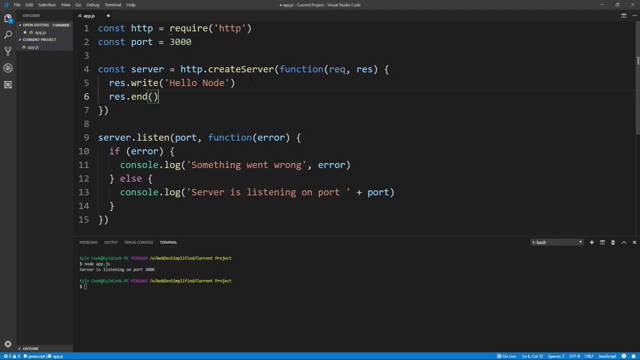 we need to do in order to get our server actually responding to actual request. so if we save that, we call node appjs inside of our console again and then if we just open up a browser and we go to localhost 3000, you'll see that we get. 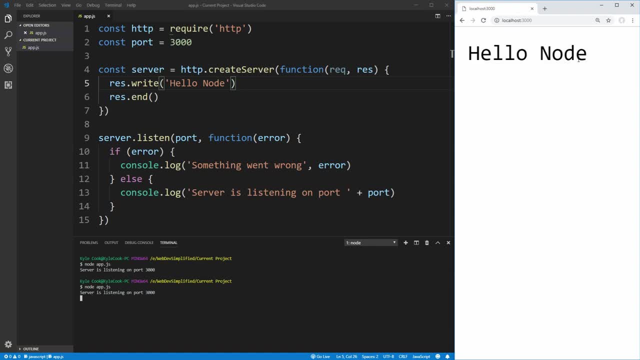 hello, load node being printed out into our browser, which is amazing, but we probably want to actually render HTML from our web server rather than plain text, so let's get started doing that now. the first thing we need to do is create an HTML file that we want to render, so let's just create a new file called 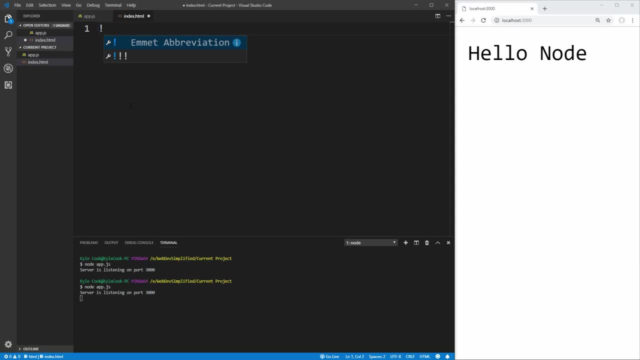 indexhtml and in VS code, if you just type an exclamation point and hit enter, it'll generate the outline of an HTML document for you, and then inside of the body we can just put this is HTML, so that we know that this is the HTML file that we want to render, and then inside of the 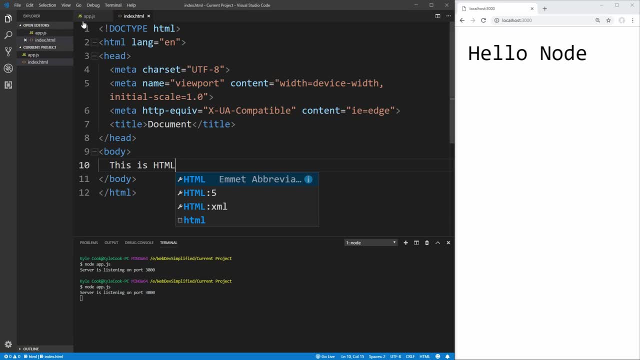 body we can just put: this is HTML, so that we know that this is the HTML file, that we know that we're actually rendering HTML here instead of our plain text back in our appjs file. we need to change the function here that we're calling with. 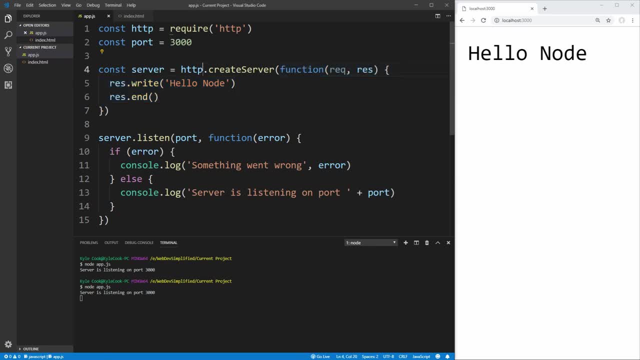 each request to tell it to send HTML instead of this plain text of hello node. so the first thing we need to do is tell the browser that we're going to be writing HTML. to do that, we'll call the write head function, and the first parameter of write head is the status code of this operation, and 200 is a good 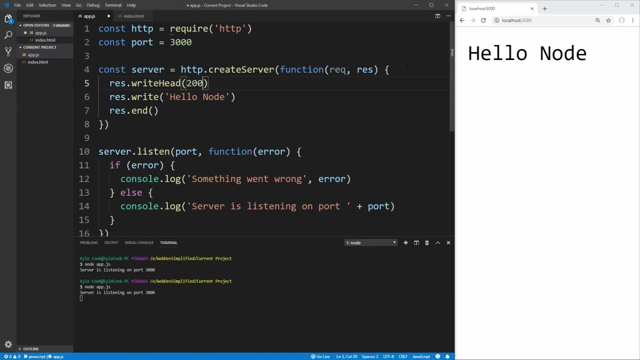 status code. it means everything went fine. so we're going to use two hundred, which indicates that everything went okay. and then the next parameter is going to be the different headers that you want to set, and one of those headers is called content type, with a hyphen in between content and type, and that is. 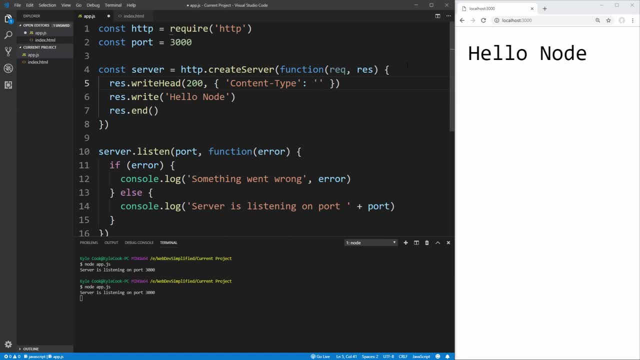 going to be the key of our object, and then the value of that object is going to be what value we want to set to that header. and in our case, we're using text slash HTML, and this just tells the browser that the information that's being sent to it is an HTML document, so it should parse it as HTML. 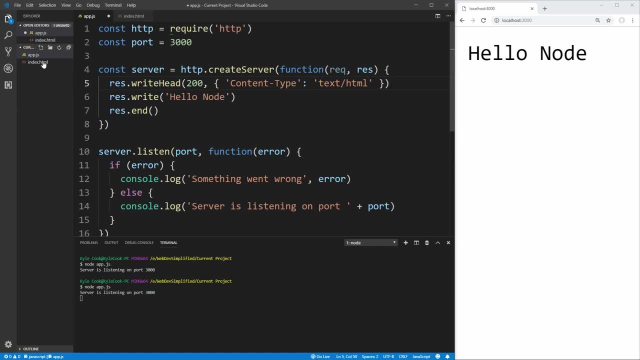 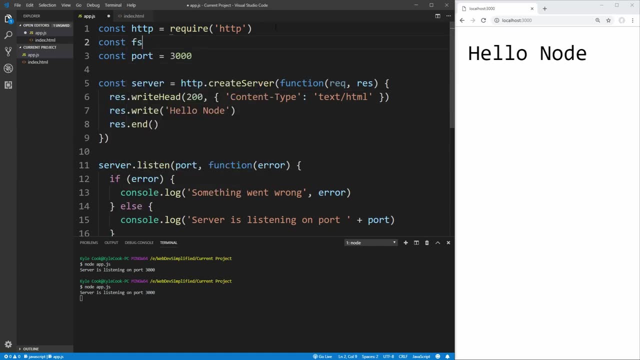 then we want to read the file indexhtml that we created earlier. so we need to import another library into our appjs and this is going to be called FS, and we just require that library, just like this, and now we have a variable called FS that has all the file handling that we need to be able to do so down here in. 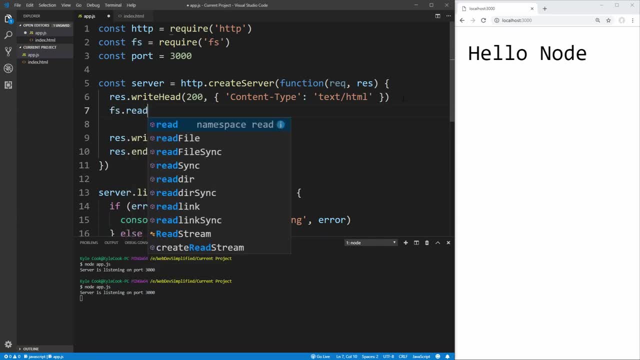 our appjs. we're just going to call the read file function of FS and this function takes the name of the file we want to read, which is indexhtml, and then it's going to take a function which is going to have an error property- if an error happened- and a data argument which 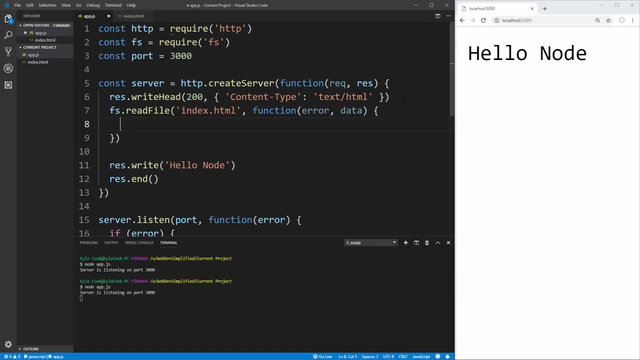 is going to be all the data from inside of that file and in here. what we want to do is, first, we want to check if there's an error, because if there's an error, we want to tell the browser that we couldn't find what we were looking for. 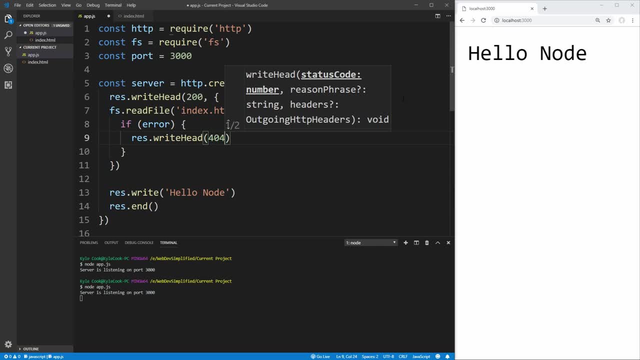 so we can say: write head with a status of 404, and 404 it just means not found, we couldn't find what you're looking for. so that's how the browser knows that is unable to find this, and then we can use our write method that we talked about.